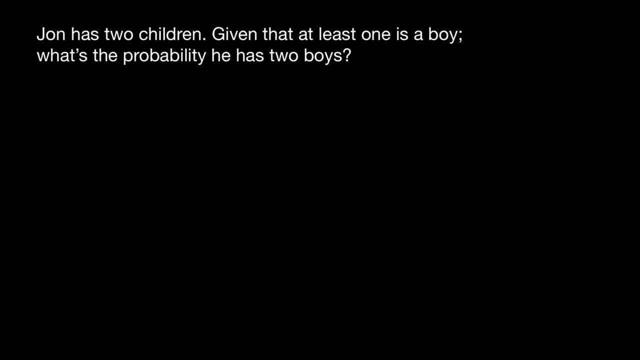 Hello and welcome to Nikolai's Genetics Lessons and today's problem seems like very easy, but believe me, many of you can make a mistake solving this problem. Here is a problem. John has two children. given that at least one is a boy, What is the probability he has two boys? First, let me 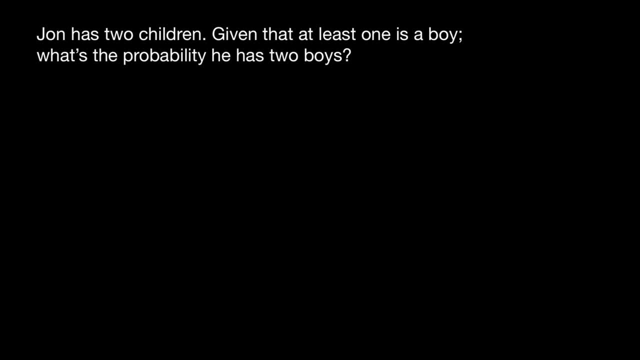 explain the common mistake that people usually make. So they think that if John already have a boy, then a probability that the second child would be also a boy would be. once again, in a family there can be only a boy or a girl, so probability is 50 percent that this is going to be a boy and 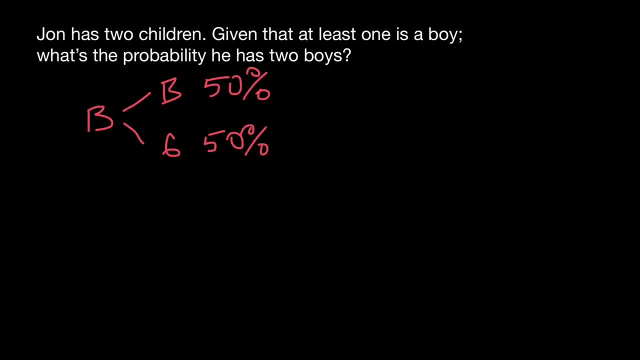 50 percent probability that this is going to be a girl. or we also can say 0.5 and 0.5, or one half and one half. This is wrong solution. Now take a look how family may have two children, so it can be a boy and a boy. the first child can be a boy and 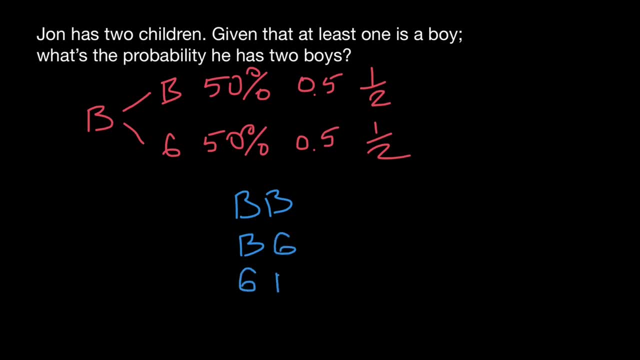 then a girl, and first child can be a girl and then a boy. and the other variant, and last variant, would be that family would have two girls and probability of each combination is going to be equal. so 25 percent, 25 percent of this combination, 25 percent of this combination. 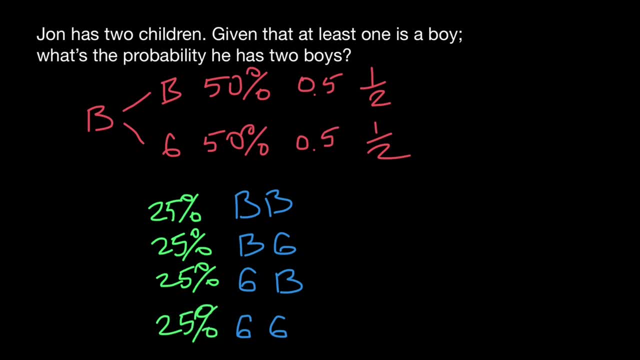 and 25 percent of this combination, or one quarter, one quarter, one quarter and one quarter. now let's read our problem again. given that at least one is a boy, will exclude this variant. so now we have three variants, and probability of each variant would be, this time, 33.3 percent. 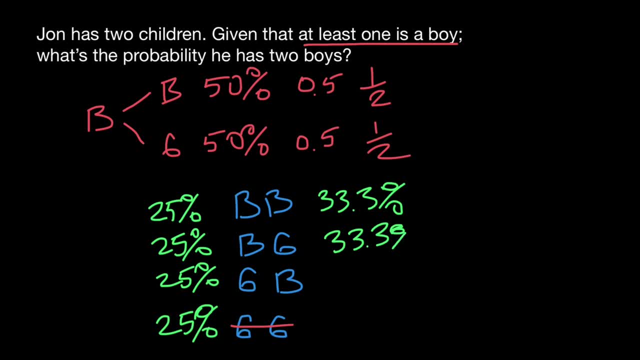 33.3 percent and 33.3 percent after we excluded this variant. we have now only three variants, and probability that the second child is also going to be a boy would be 33 percent and not one half, and this is all for today. thank you for attention. please subscribe for my new videos that i post. almost every day and see you in the next video. goodbye.